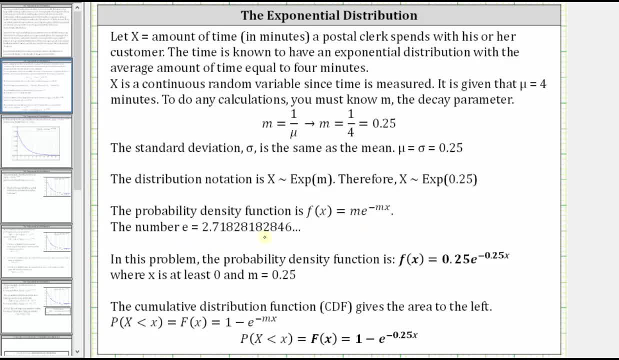 where e is an irrational number, approximately 2.718.. In this example, since m is equal to 0.25, the probability density function is: f of x equals 0.25 times e raised to the power of negative 0.25 x. 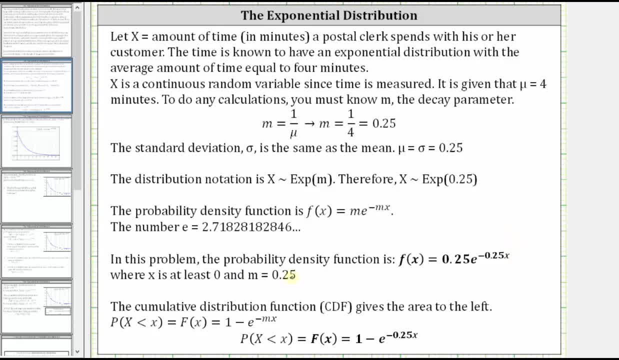 where x is at least zero and again m is 0.25.. The cumulative distribution function gives the area to the left under the exponential distribution which is given by a big F of x equals one minus e raised to the power of negative mx. 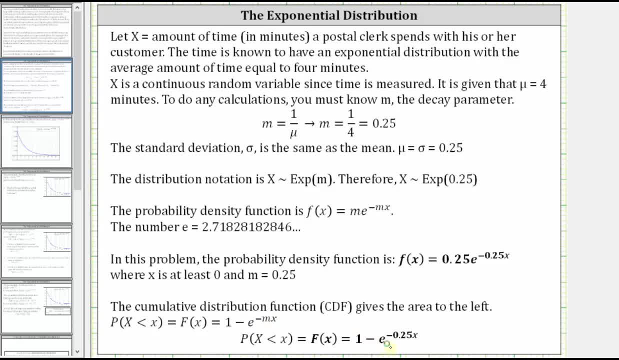 Or in our case, big F of x is equal to one minus e raised to the power of negative 0.25 x. Let's look at the graph of the probability density function, which is here on the coordinate plane. Notice how there are more smaller values. 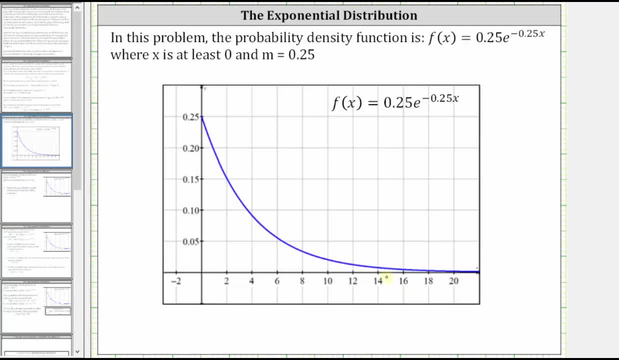 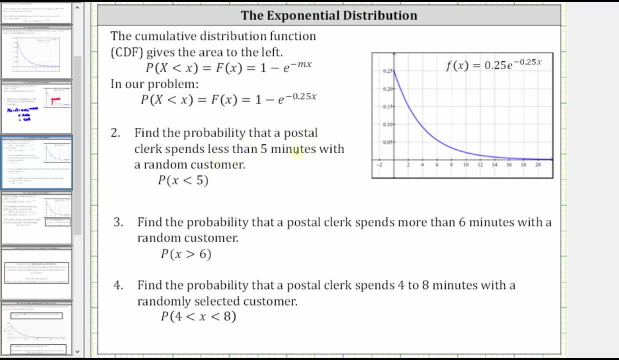 and less larger values in the exponential distribution. And now let's find some probabilities. We want to find the probability that a postal clerk spends less than five minutes with a random customer, which is a probability that x is less than five. To find this probability. 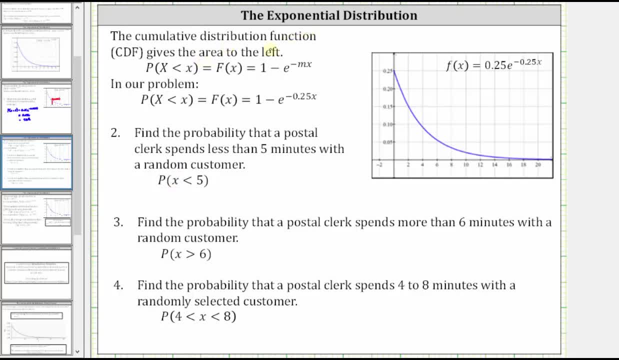 we will have to use the cumulative distribution function, which is big. F of x equals one minus e raised to the power of negative mx, And this gives the area to the left of the value of x. So for the probability that x is less than five, 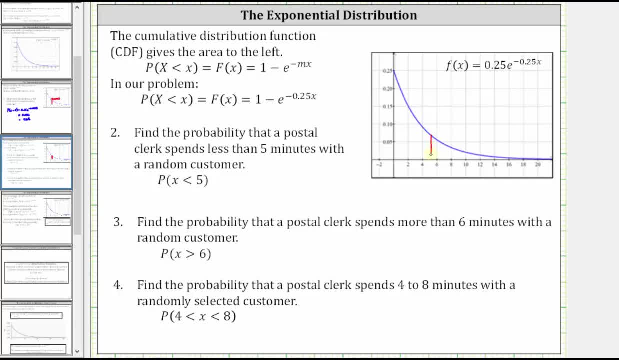 going back to the graph, here's where x equals five, because we're looking for the probability that x is less than five. we want to find the area under the curve to the left of five, which is this area here, which is on the left. 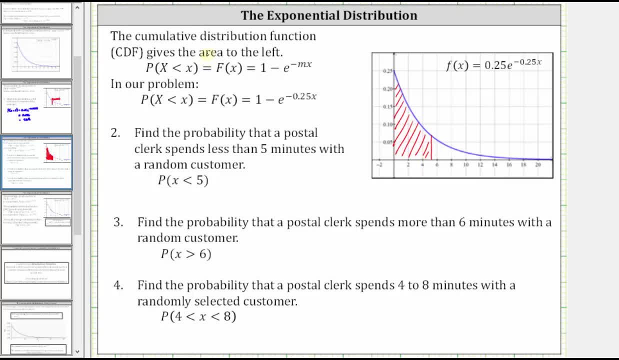 And therefore we simply substitute five into the cumulative distribution function to find this probability. So the probability is equal to one minus E raised to the power of negative 0.25 times five. Going back to the calculator, we have one minus second natural log. 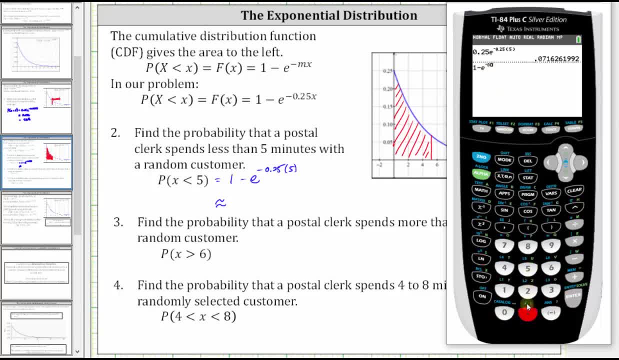 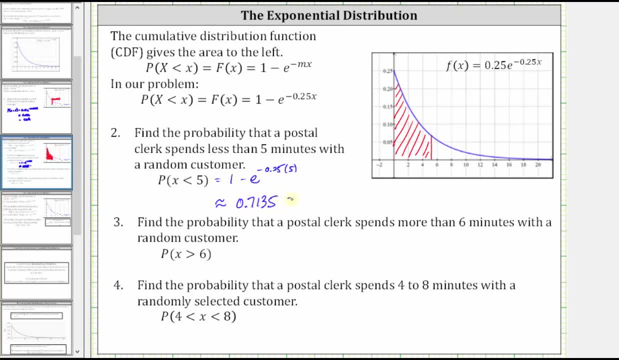 for E, raised to the power of negative 0.25 times five, Enter To four decimal places, we have approximately 0.7135, which is 71.35%. For number three, we're asked to find the probability that a postal clerk spends more than six minutes. 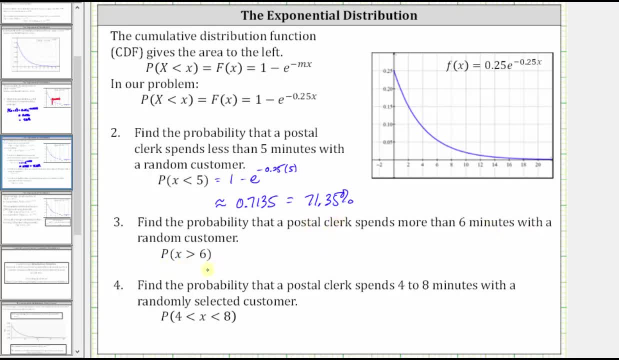 with a random customer, which is the probability that X is greater than six. To find this probability we need to find the area under the probability density function. So here is: X equals six. The area on the right. this area here is equal to the probability that X is greater than six. 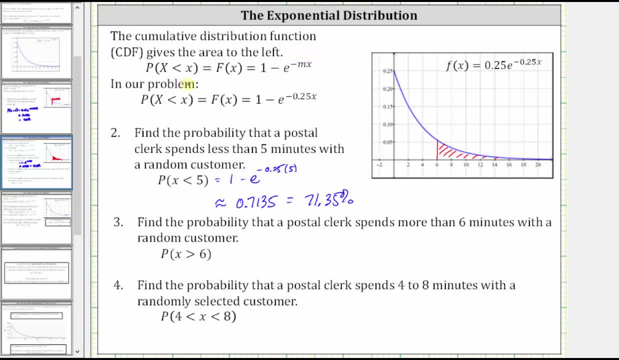 But remember, the cumulative distribution function gives the area to the left, not the right, And therefore to find this area we will have to find the area under the entire curve, which we know is equal to one, this area here- and then subtract the area to the left of six. 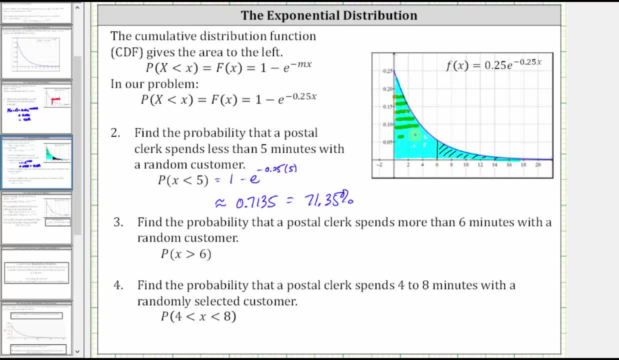 which is this area, which will leave us with the desired area, which is the area to the right of six. this area here, So the probability that X is greater than six is equal to all the area under the curve, which is equal to one minus the area. 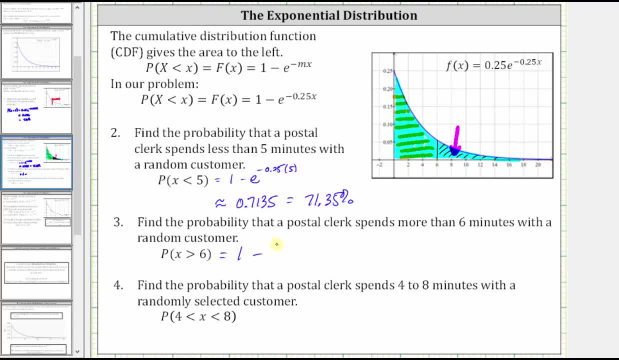 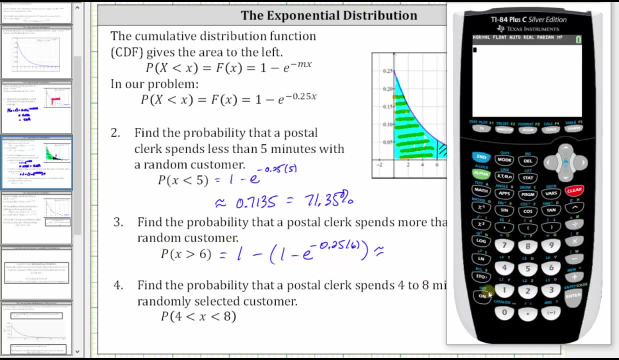 under the curve to the left of six, which is equal to the quantity one minus E, to the power of negative 0.25 times six. So now we'll go to the calculator. We could simplify this expression, but we'll go ahead and type it in just like it looks. 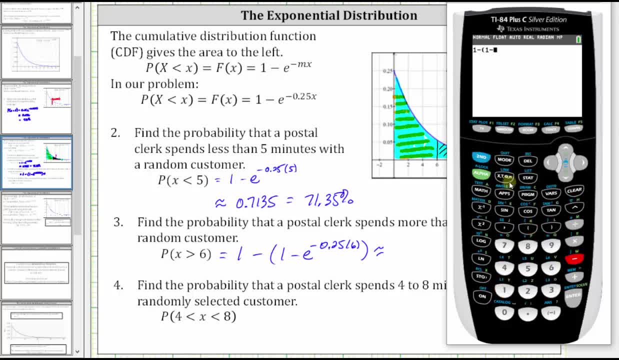 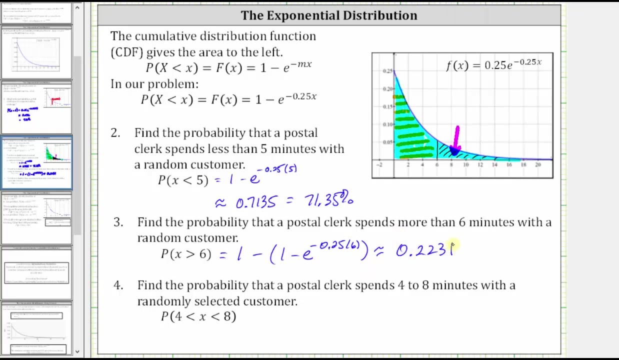 One minus open parenthesis, one minus second natural log for E to the power of negative 0.25 times six. Right arrow close parenthesis enter To four decimal places. we have approximately 0.2231, which is equal to 22.31%. 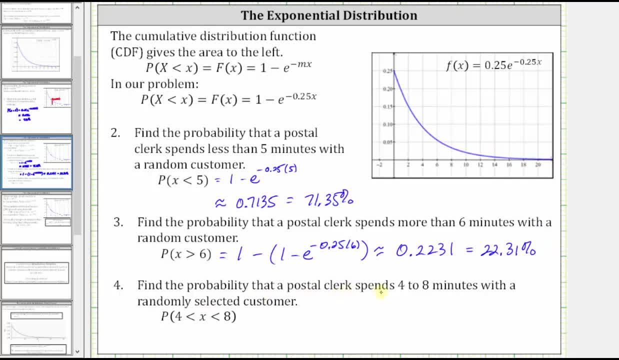 For number four, we want to find the probability that a postal clerk spends four to eight minutes with a randomly selected customer, which is a probability that X is greater than four and less than eight. Let's go ahead and shade the area under the curve between four and eight.